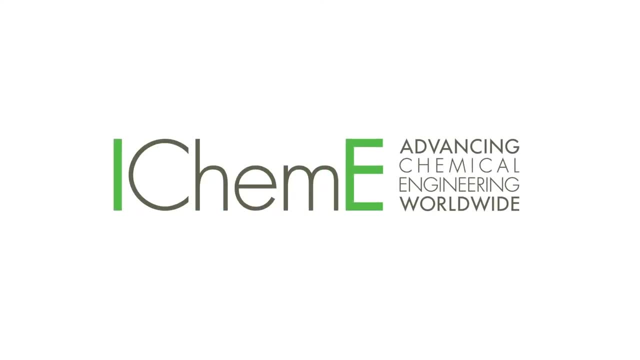 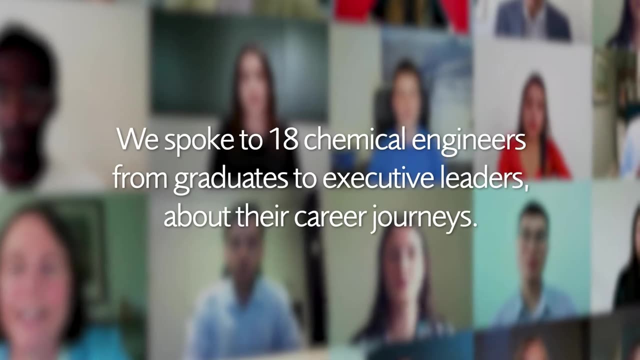 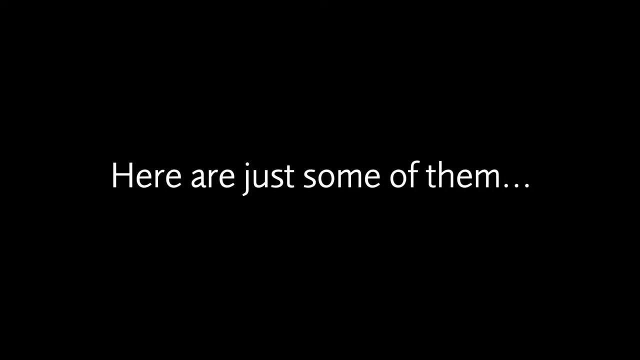 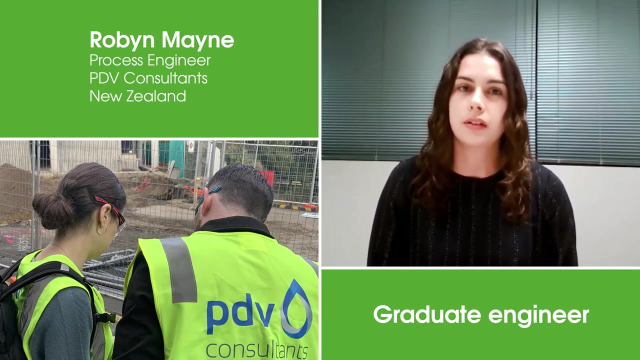 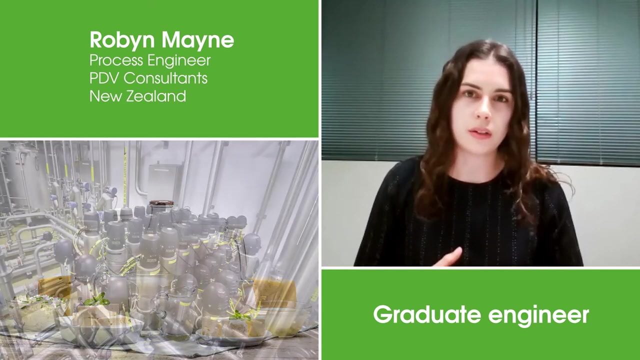 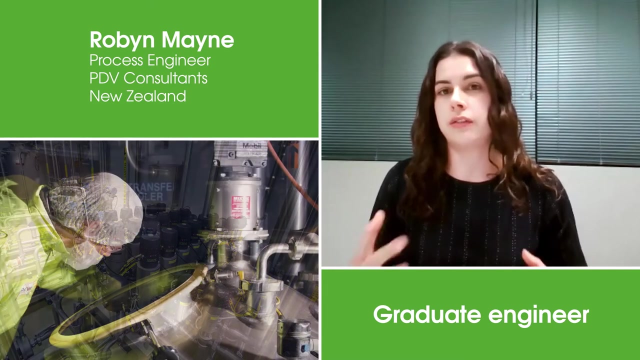 At PDV Consultants, we work on process and manufacturing projects in the dairy industry. Advice that I would give to students currently looking for a graduate role is to not be afraid to apply for internships rather than graduate positions, because internships are a really good opportunity to give you an idea of what the job's actually going to be like. 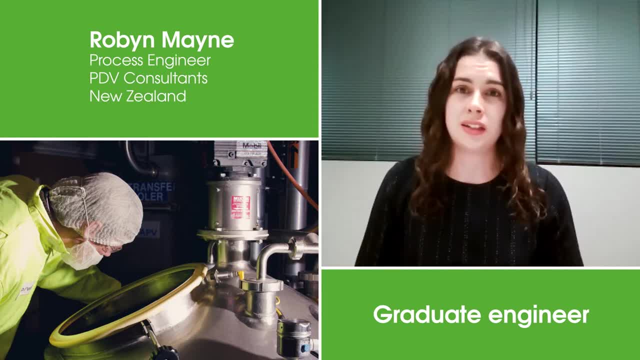 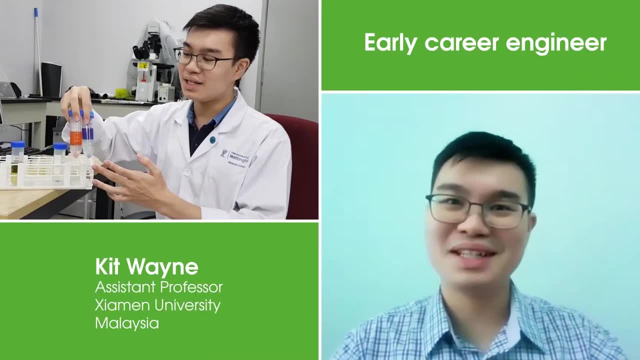 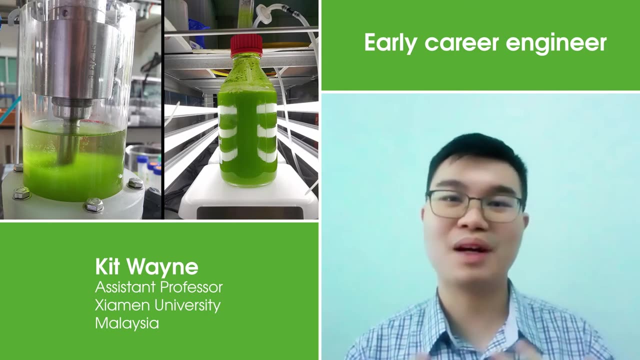 and it's also an opportunity to make good connections in the industry as well. My greatest achievement so far, in my opinion, is the research that I've developed, So I've come across new systems which I can help to cultivate microalgae in a more higher efficient manner. 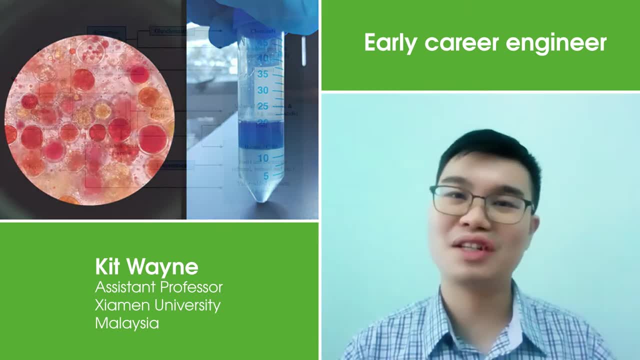 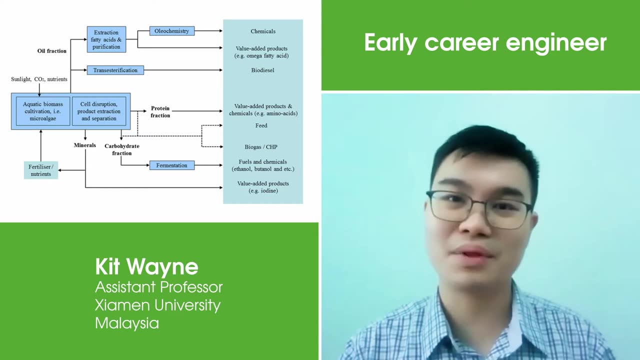 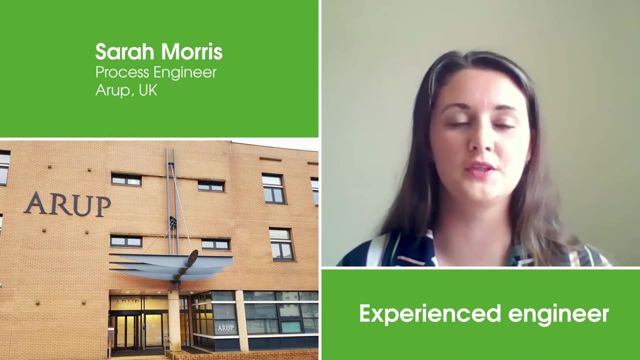 and I also developed this noble multi-phase partitioning technique, which has been proven to be able to extract not only one product but multiple products in one single processing system. I work in a range of different aspects of wastewater and clean water design. My advice to a student doing an application is: 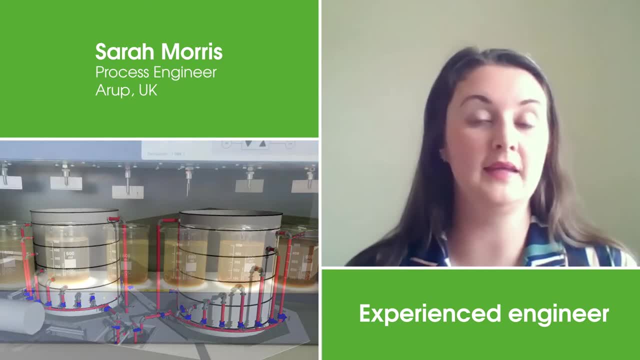 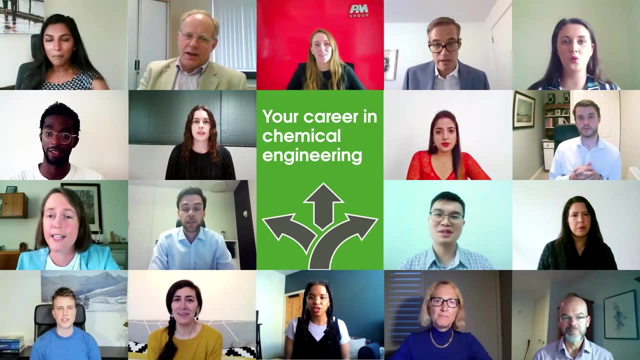 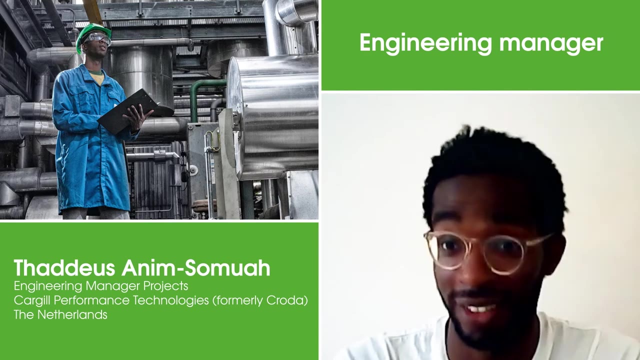 think about your skill sets outside of academia. If, for example, you're part of a sports team, talk about teamwork and your commitment to that team. My best advice to students looking for a graduate role is to first understand yourself. What drives you, What motivates you? What are you good at? 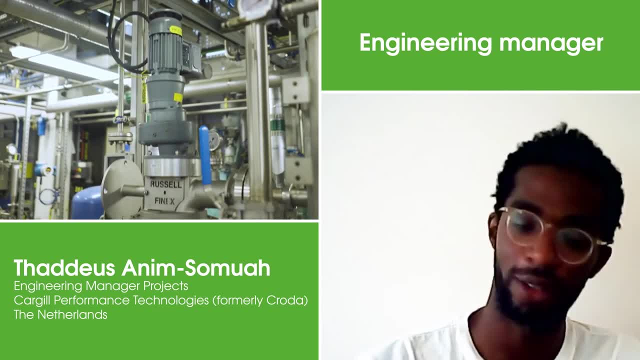 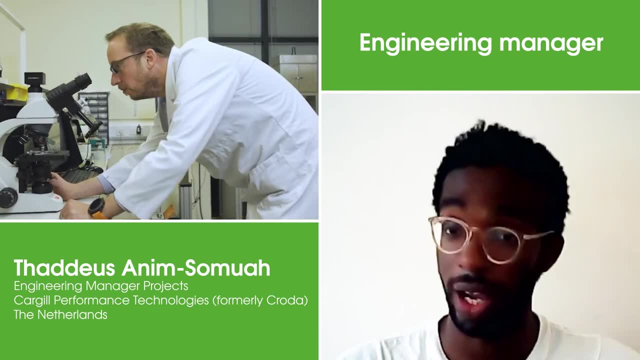 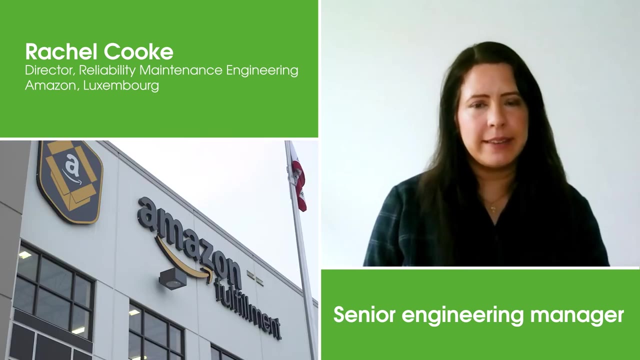 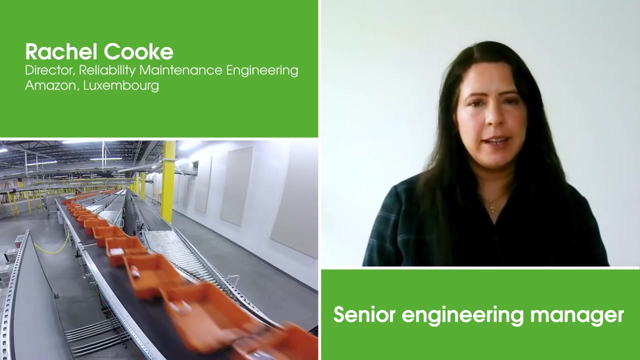 And when you understand this, then you look as well at the opportunities out there in an industry and you can see what you know what kind of matters. In my role, I lead a team of approximately 70 people based in eight different countries across Europe, and we set the reliability strategy, the maintenance best practices and general knowledge. 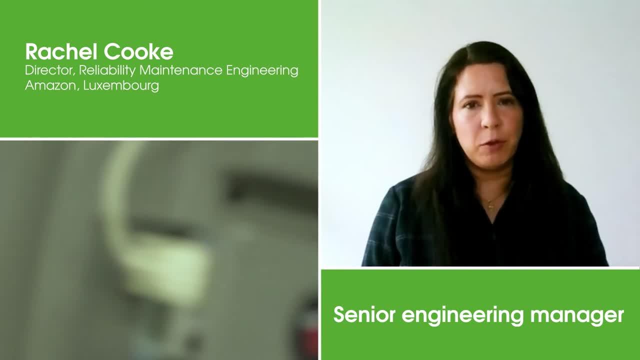 sharing across Amazon to ensure that all our equipment runs reliably and smoothly. I've had many mentors throughout my career and it's been a great experience for me. I've had many mentors throughout my career and it's been a great experience for me.